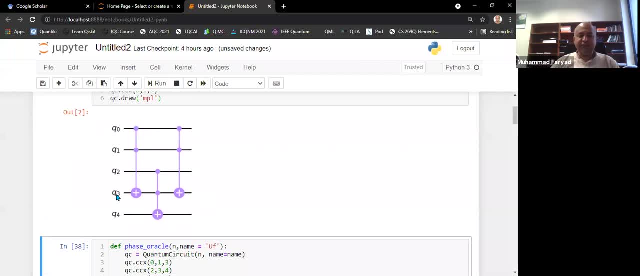 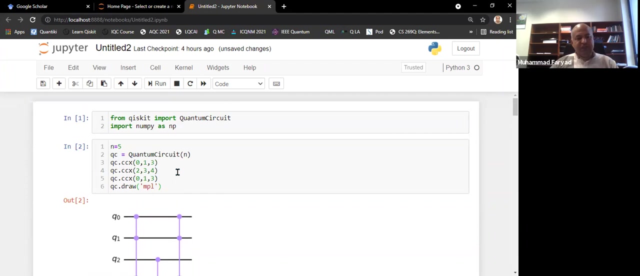 qubit That is set in that I will set in zero state later on And this Q4 is my qubit that I will set in the minus state. So this essentially implements CCC x kit, where this Q3 is that auxiliary qubit that will be set in the zero state. And you know this. if I use later on this as a Grover, you know Oracle. so this will essentially implement CCC x kit. 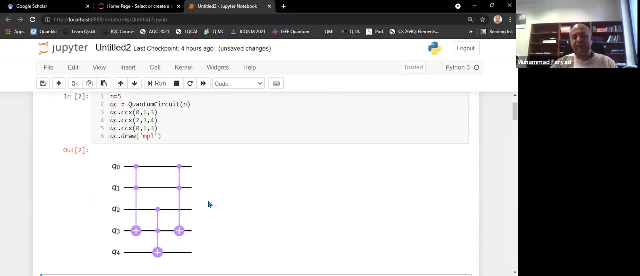 this will essentially mark 111 element as the answer of this problem. If you want to mark, let's say, 101 element, so then what you will have to do, that's a 101.. If that's what you want to implement, I will need this q1 to first have an x gate. So q, c, dot, x and bit number. 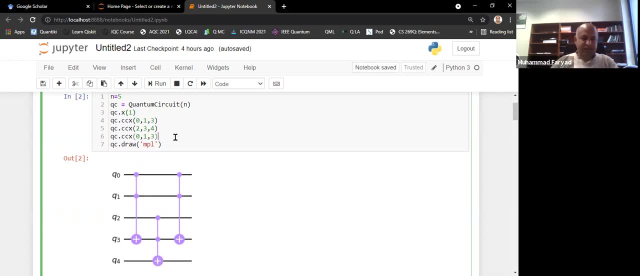 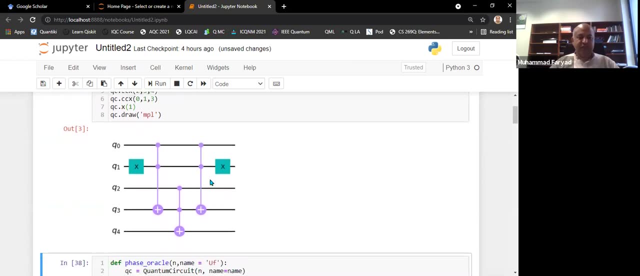 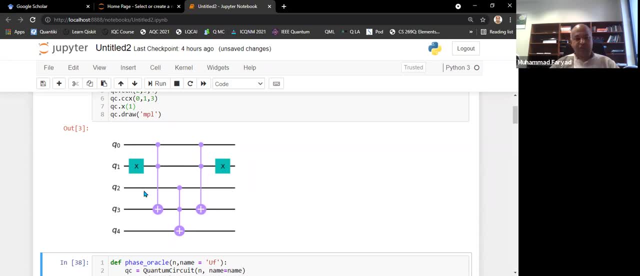 And it will remain 101 at the output. So this, you know, implements the Grover article for 101. And since you remember from the class that sometime we have to repeat the Grover and the diffuser part again and again, so I'm not going to put this into a function. 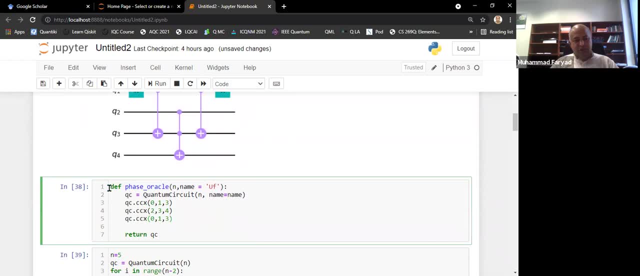 So for that you can do, using this, this, you know, function definition, So I'm defining, So I'm defining, So I'm defining this phase oracle function. It has this n as input, So n is the number of qubits, And then optionally, I can you know, set this input name to some uf. 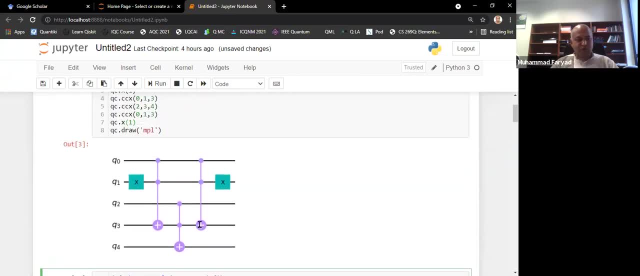 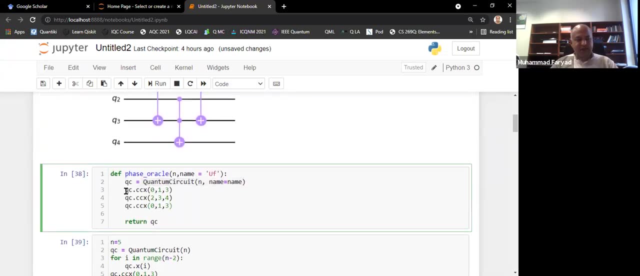 And now I initialize this quantum circuit And if you want to, you know, use this, this one, this 101, as the marking for this. let me replace this 111 with this. So now, this part is, you know, part of this function. wherever I will call phase oracle, this phase oracle will essentially call this circuit. 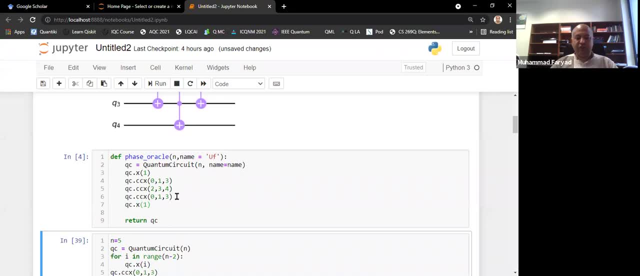 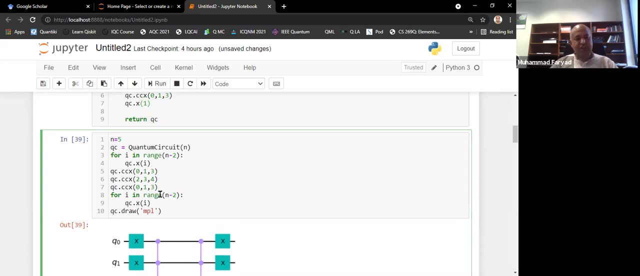 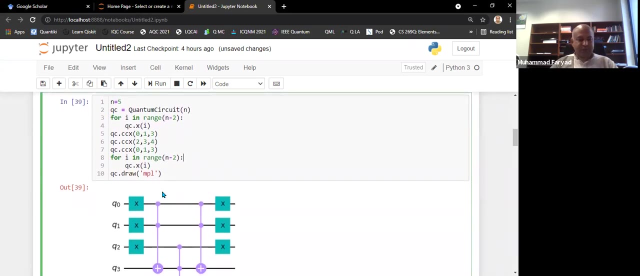 So since this is a function, I don't see any output here drawn. Similarly, this is a function that I have made to represent the diffuser part. So if in the In the diffuser, if you remember, we had the Hadamard layer, then uf0, and then the Hadamard layer again. 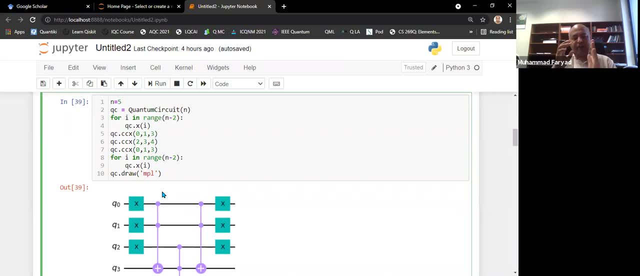 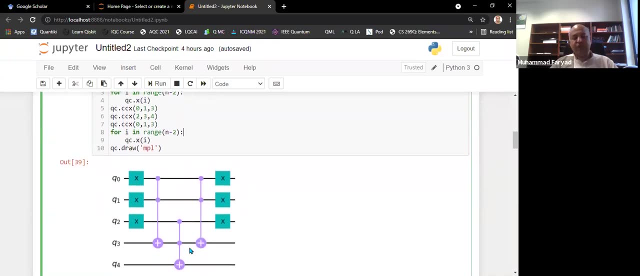 So this uf0 has to mark 000 element. So this essentially, you know, implements the 000 control gate, because this q0, q1, q2 have this x gates, So this control gate would be initialized by 000.. 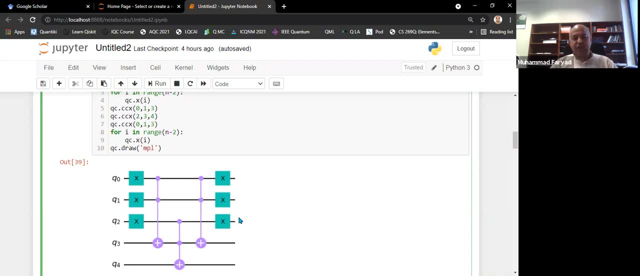 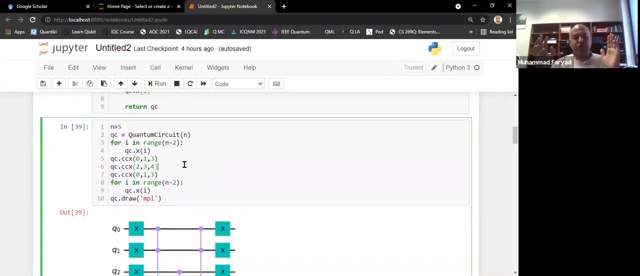 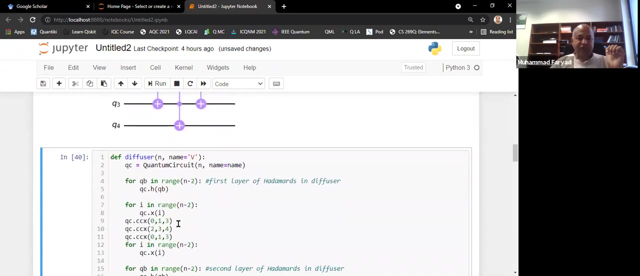 And then this 00 will be turned into the same 00 as well by these x gates. So this circuit remains fixed throughout this, you know, Grover set because only 0th element has to be marked. So let's run it. So this is the one, And then I put it as part of the diffuser circuit. 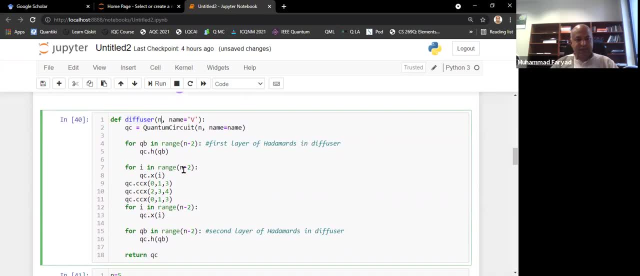 So my diffuser function has this n as input and its name is v, And now I have a quantum circuit with n qubits. So- and I will later on Set to five- And I have this layer of Hadamard. I just apply Hadamard on the first three qubits. 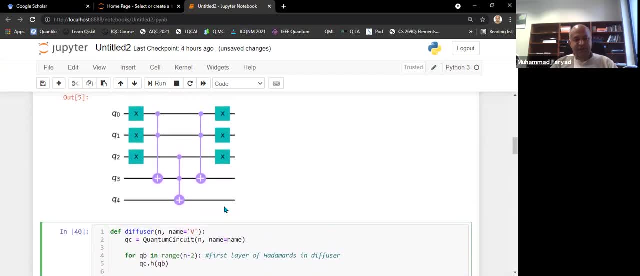 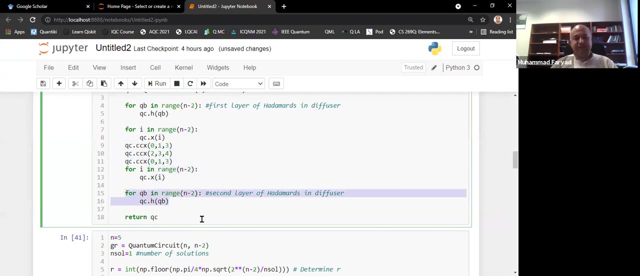 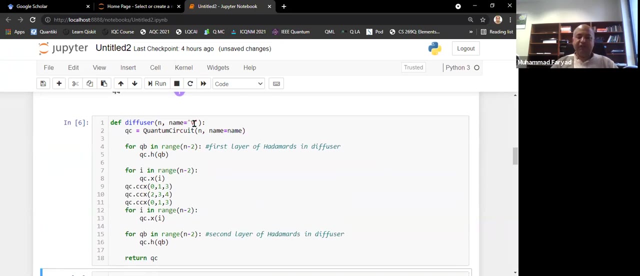 And then this is the same circuit that is printed over here, which is essentially marking the 0th element, And then there's this second Hadamard layer, And then, you know, I return qc. So this function, whenever it is called, will implement this diffuser v. 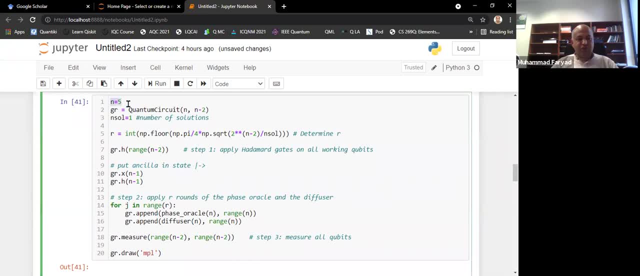 Okay, this is now my main program. You see I have. n is equal to five, So there are total five qubits. Three are the working qubits because it's going to be a 3 qubit Grover algorithm. And then there is the fourth qubit which I have to put in zero or for the sake of implementing, you know, the Oracle. 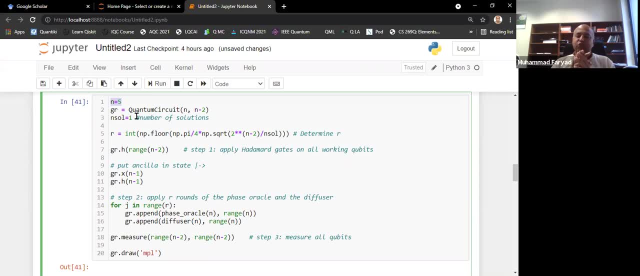 And then there is the fifth qubit, which is again the encilia qubit, that I will have to put in the minus state: N is equal to 0, and d is equal to 0.. And d is equal to 0. 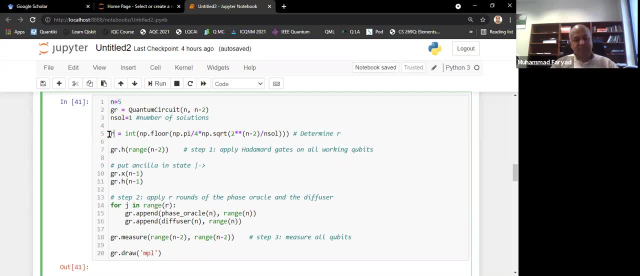 now, before i- you know uh- run this algorithm, i have to find this r, and r is the number of times i have to implement the iteration of grover, you know operator, and this is uh, if you remember, is was pi by 4 divided by, also, square root of capital n, and capital n in this case is 2, power and minus. 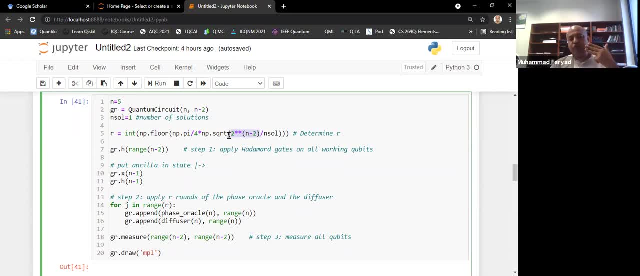 2. so n is 5, but there are only three working qubits, so it's two power three, and then this number of solution is that mu that we were talking about last time, so let me actually write this as mu. i think you will be able to relate it with the 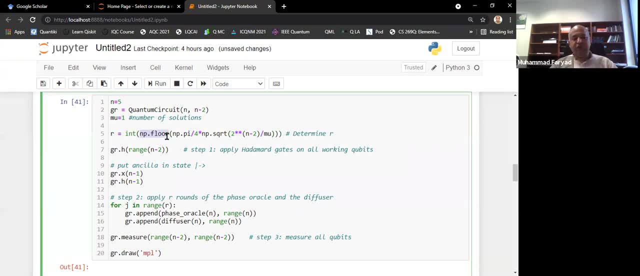 answer. and then over here i have this flooring function, because if it is a non-integer function, like 3.7, something like that, then i will floor it to 3 and take its integer part, uh, as my value of r. okay, now, once i have r, i first need to apply this. hadamard transform the. 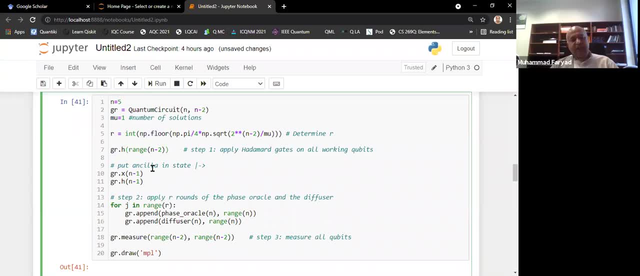 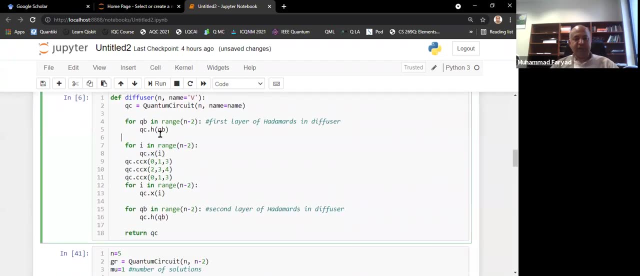 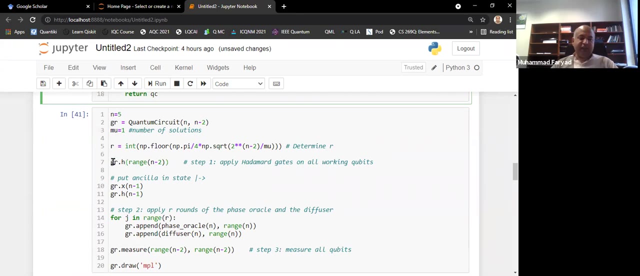 first step of the grover circuit. and one way of doing it is: you know the loop just as you know we did here or we did here. but this is just another way. this is syntactic sugar in later in python that i can also implement the loop. 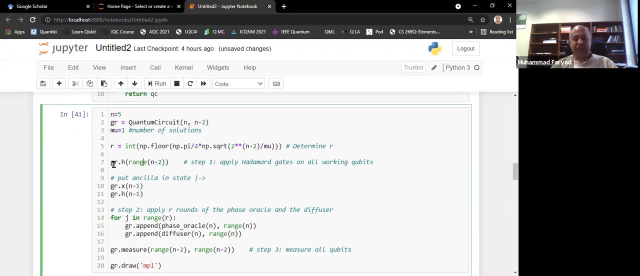 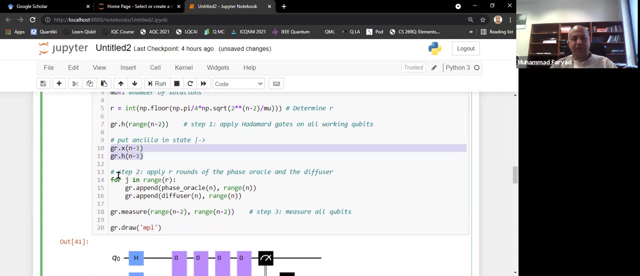 you know, using this range function, so gr dot h, like hadamard gates on this grover circuit, so by specifying range of three. so it applies, you know, for from zero to three minus one. okay, so now here i am putting my last qubit in the minus state, by first applying x gate and then 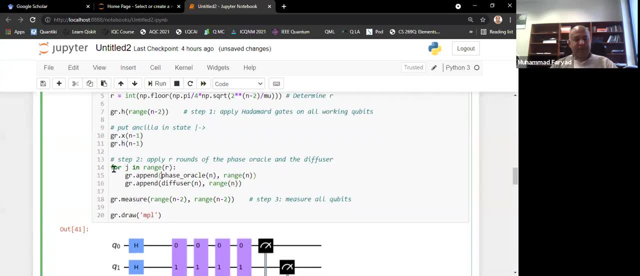 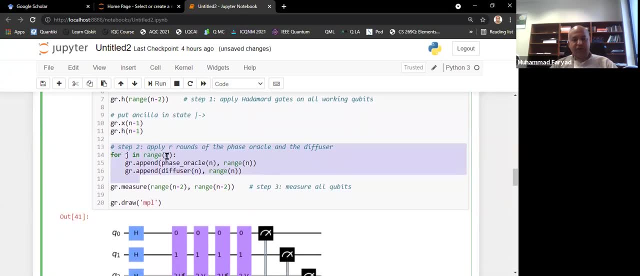 the hadamard gate. and then this is the main, you know, central part of this algorithm for j in range r, i first append my circuit with the phase oracle and it. it takes n qubits and then i give this range n because you know, this gr is a circuit that has qubit zero, one, two, three, four. 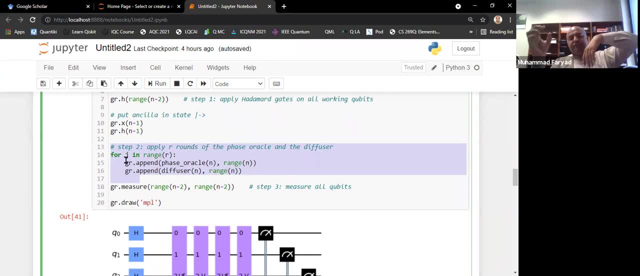 and then when i give an append command and i ask another circuit you know to be made part of this, i have to specify that uh, what are the qubit you know, what are the qubits you know that are in the you know arrangement that has to be connected with that. so this range n tells uh this append. 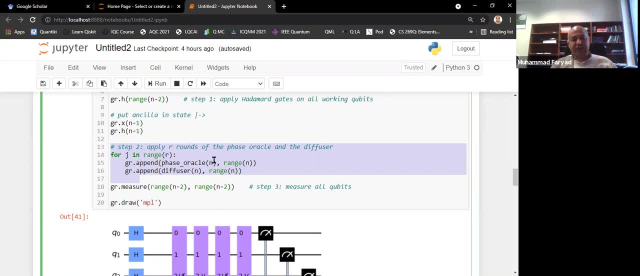 command that you append this phase article uh that has this n qubit uh, so that the zero one, two, three, four qubit go to this uh in in this order of zero one, two. you can actually change the order here as well when you're appending. for example, you can connect: 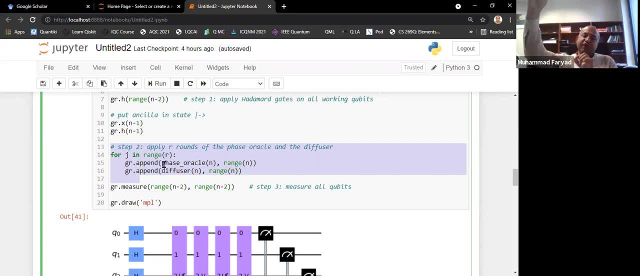 fourth qubit with the first qubit of the circuit that you're appending, and so on. but here i'm appending in the, you know, straightforward order. so that's why range n, range n. similarly, i append my diffuser and now, once we have, you know, implemented this grover for as many time. 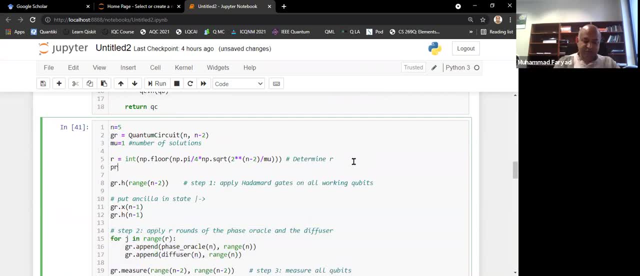 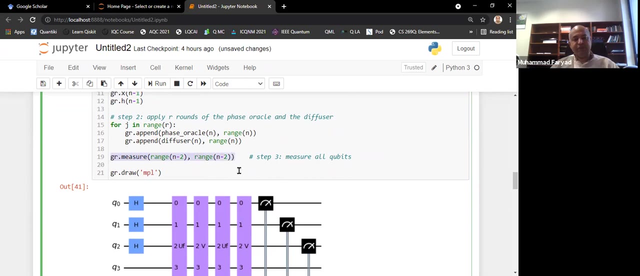 as we want. let's actually print r here so that we know what is the value of r, all right, and then at the end i just have these measurements, okay, so i apply. so again, you see, i'm applying these major gates using this range function. so 012 quantum qubits are being 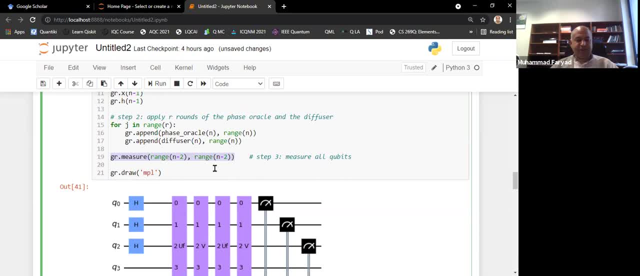 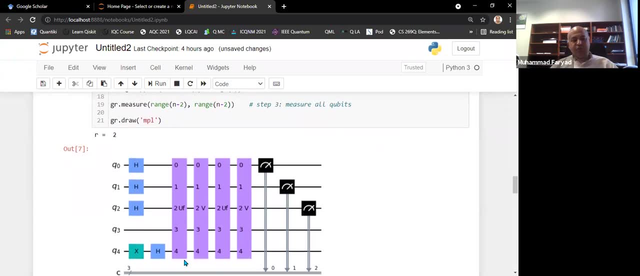 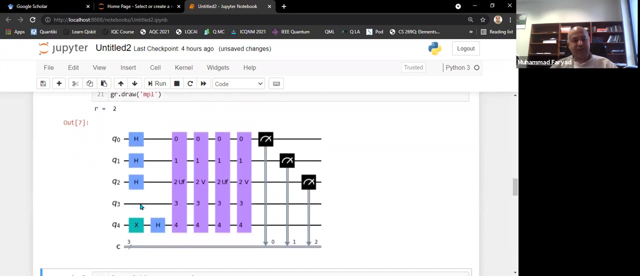 measured and put on 012 classical measurements, and then there's this draw circuit. so let's run it okay. so we see r was computed to be 2, so that's why this u and and ufnv- ufnv, appear twice. now you can see there's this first layer of hadamard. nothing is has been. 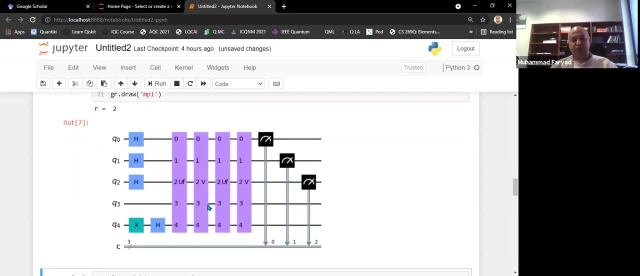 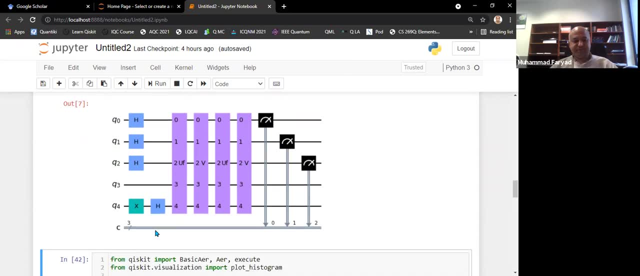 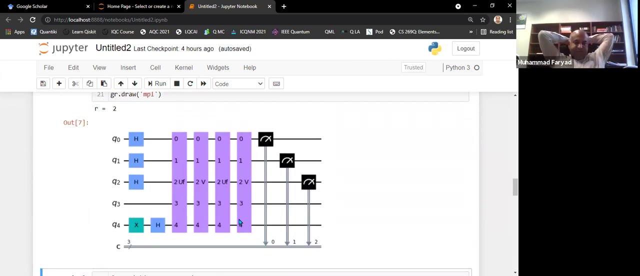 done to q3- this is qubit- remains in zero required for implementing oracles in ufnv, and then this q4 is put to this minus state. okay, so any question about implementing this circuit, sir, out of the five qubits, we always have to work with the three qubits. is this the general rule or specific for this problem? 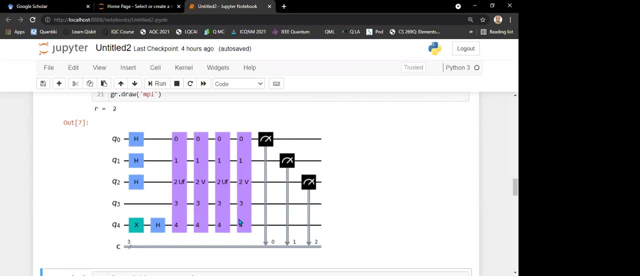 what do you mean by general rule? here we have five qubits and we are working with three only, right, so if we have n, so we will be working with n minus two, always. no, no, no, it depends. you see, you decide number of qubits by first deciding how many are the qubits. 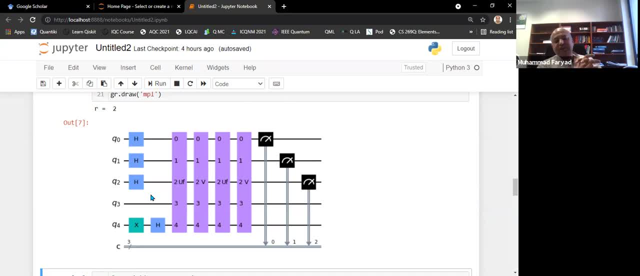 are the you know search items in your search database. for example, you have eight elements in your search database like capital. n is equal to eight. so it means you need three working qubits. right, small n is equal to three. so for three working qubit i have to implement the oracles and 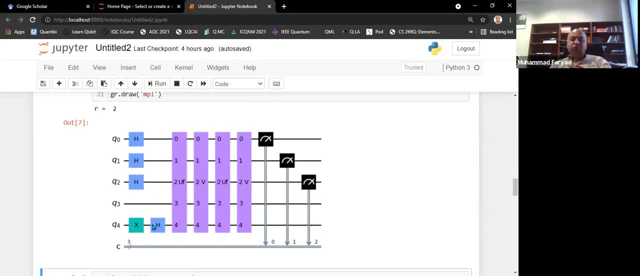 to implement the oracle i needed two auxiliary qubit, because we just saw in the presentation before that to build a three qubit oracle i need uh two, uh two qubits to implement the oracles and auxiliary qubits. so one was set in zero and the other was in minus, so i need five qubits. 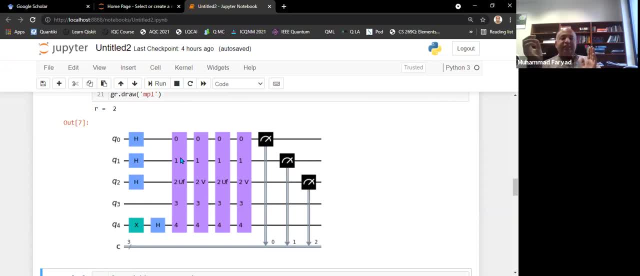 now, if you want to work with a search space that has 16 elements, it means you need- n is equal to four. you need four working qubit. so if you have four working qubit, you will probably need three qubit in zero state and one qubit in minus state. so four, three plus three plus one you will need. 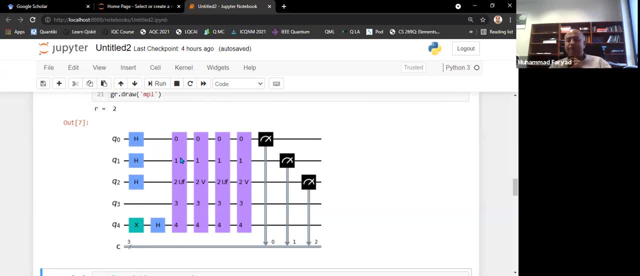 eight qubits to work in total. okay, that's another question. and can we use this algorithm for finding eigenvalues of the matrix, or we can we solve the polynomial equation with this one, this grover algorithm? yes, not directly, unless you can convert that problem into a search problem. 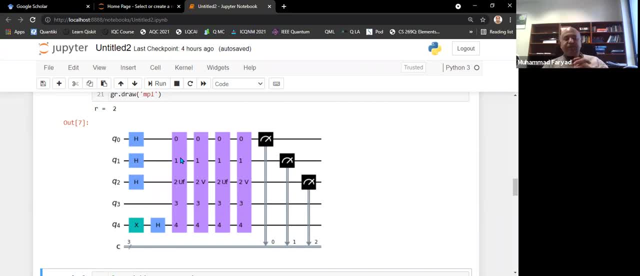 and implement on oracle. that, you know, gives a phase value when the solution of that problem is found. oops, okay, and you see i have selected a problem which has three working qubit for a reason, because this is restricting my total number of qubit to five. and you have seen, uh, yesterday that most of the ibm quantum computers 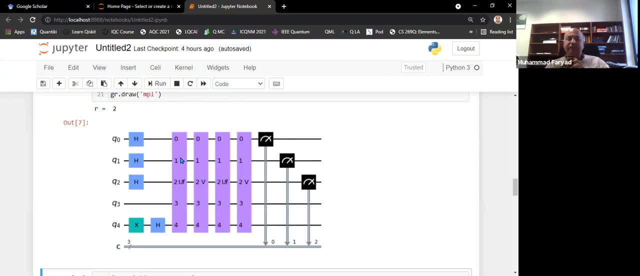 uh, at this at the lower end has five qubits and they are easily available. uh, if you go to, let's say, six or seven qubit, you will need a higher end quantum computer, and then most of the high-end quantum computers are not even actually available freely. so 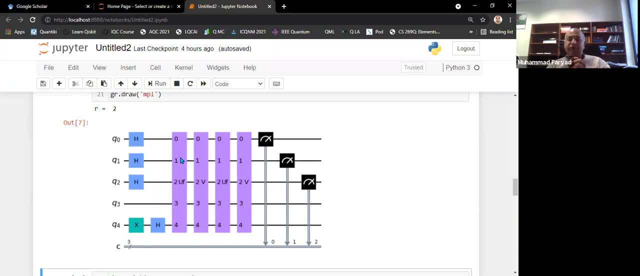 So most of the algorithm that we plan to run on a quantum computer, we try to keep the number of cubits towards the lower side because we are in the class we're just learning, you know, to, to understand algorithm and to implement it. 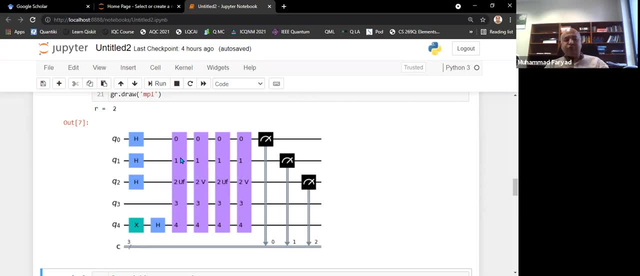 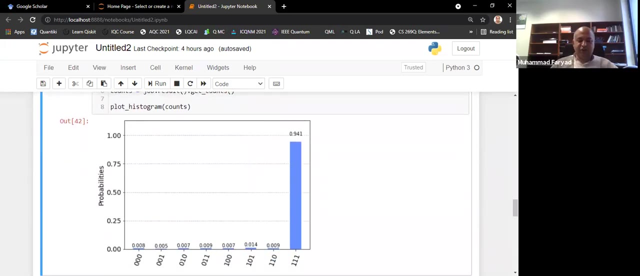 If you have to solve some practical problem, then we can decide to go with higher number of cubits. Okay, Yes, Thank you. All right, So let me run this. uh, you know circuit I, before this problem, I had, you know, a. 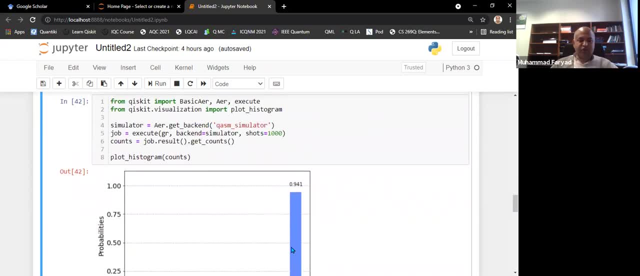 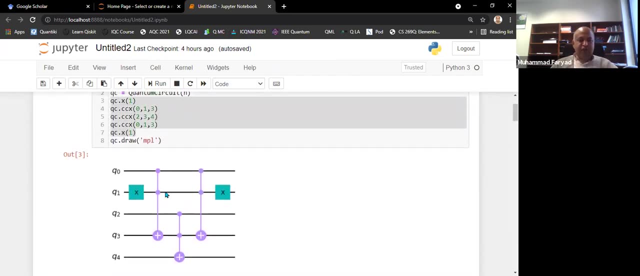 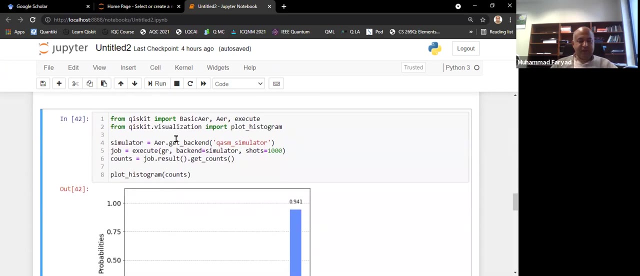 zero. mark one, one uh as uh. my answer So this: these are older simulation results, but no, we have more: mark one zero, one uh as the solution. So we should be, you know, getting one zero one with the high probability. 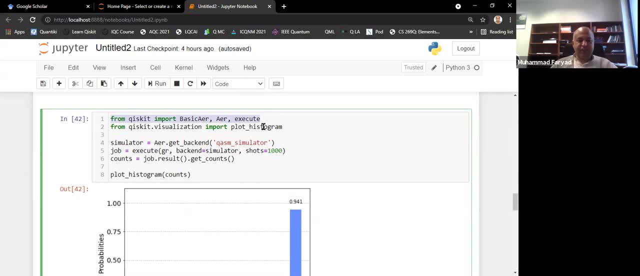 So again for running, you see, from Kisket I import basic area, execute, plus histogram et cetera, And then I select my simulator as a cost simulator and then use this command: Execute. this GR is the Groover circuit. 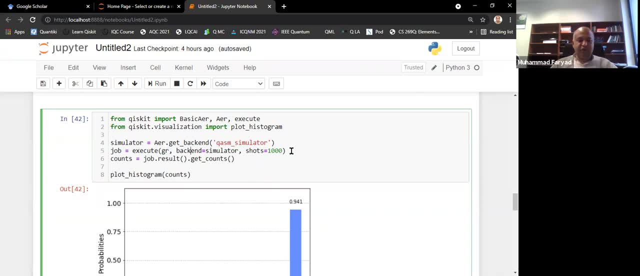 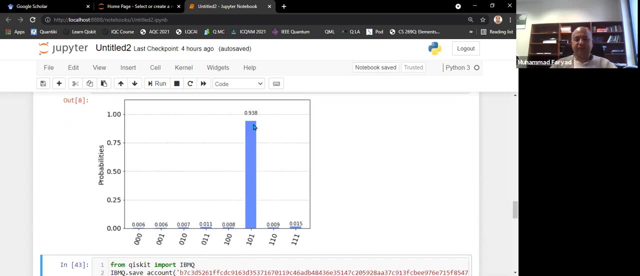 Then backend is now my simulator, cost simulator, and I'm using it for 1000 shots. So let's run it perfect. So you see, one zero one is coming with high probability, but still we are getting others as well, And this is not because of errors. 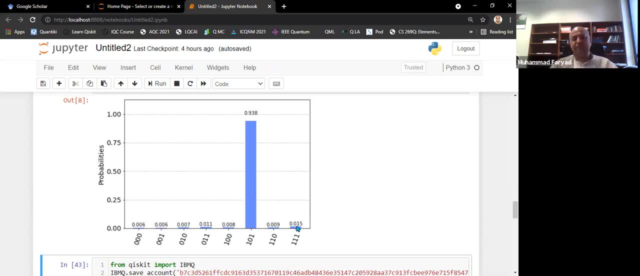 You see other states with some probability as well, And this is simply because we saw last time that, after rotating, our state may not exactly align with the solution state, As we are rotating with integer number of steps and the state could be, you know, uh. 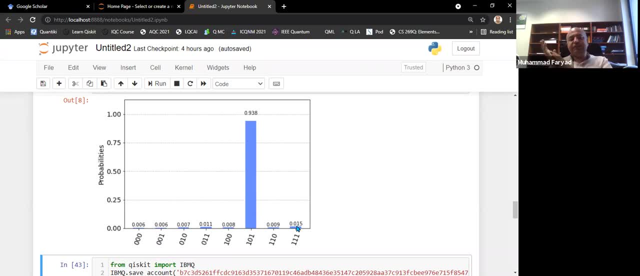 within plus minus alpha by two. So this means that, uh, uh, there's always some error in my element, because the state factor at the end is mostly aligned with the solution state. Uh, but uh, there is a small component perpendicular to that as well. 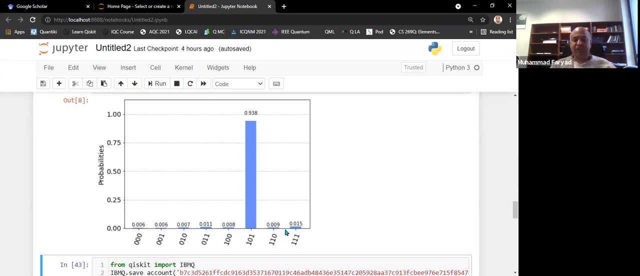 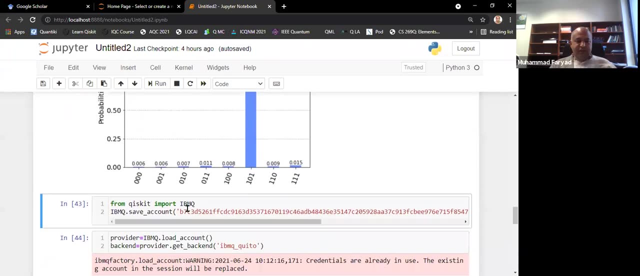 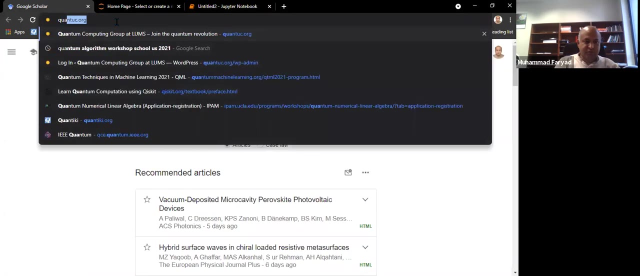 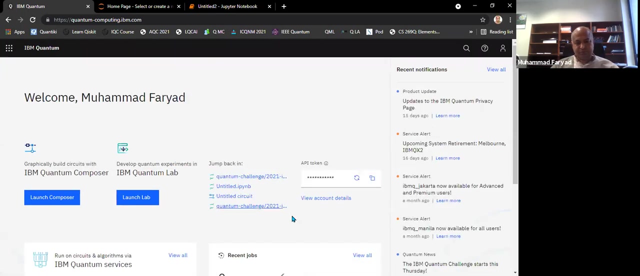 So that's why we see uh, non solution state values as well in the answer. Okay, So let me run it on the quantum computer now to see, and let's see which one is the least busy right now. So let's view them. 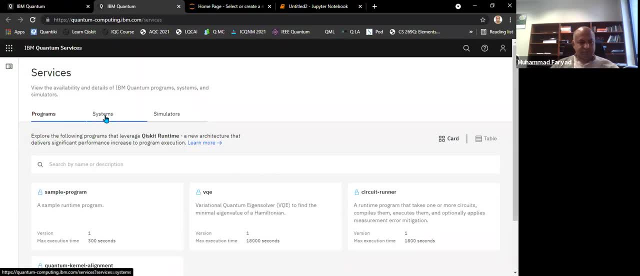 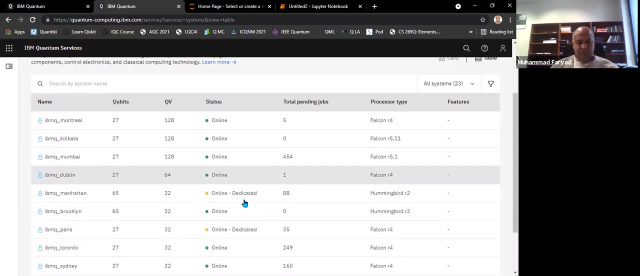 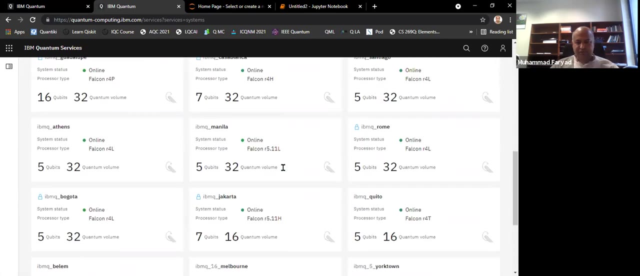 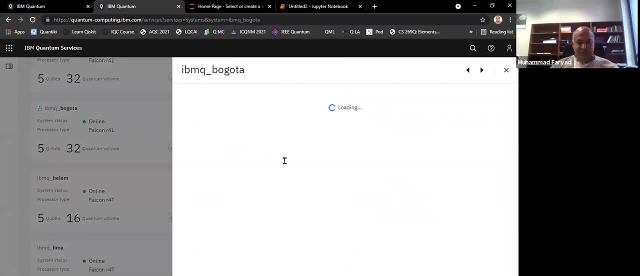 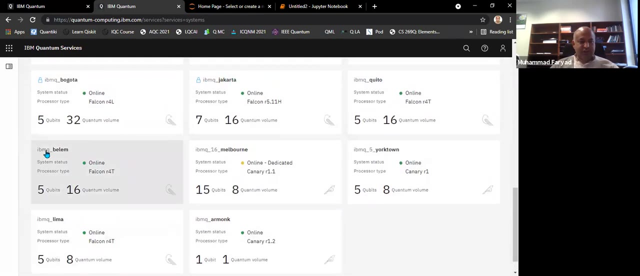 Very low quantum wanting. Let's see if this bogota Is availableиров. Bogota is 335 jobs too. Busy bellum has only three jobs, Some other. so white a K. so let's try to run on vellum, because this has a volume 16.. 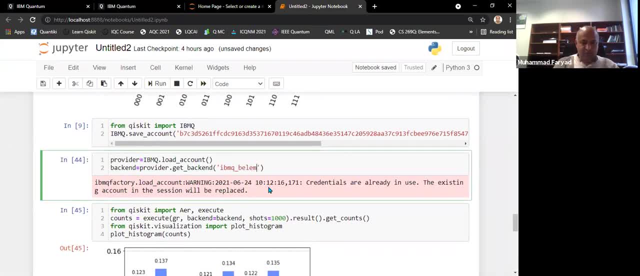 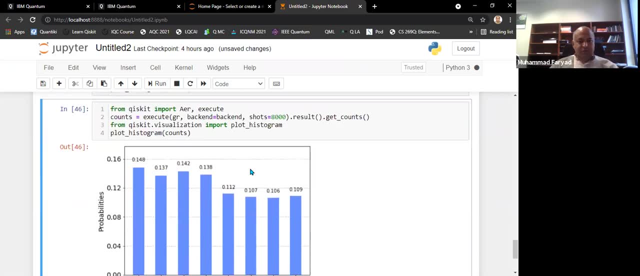 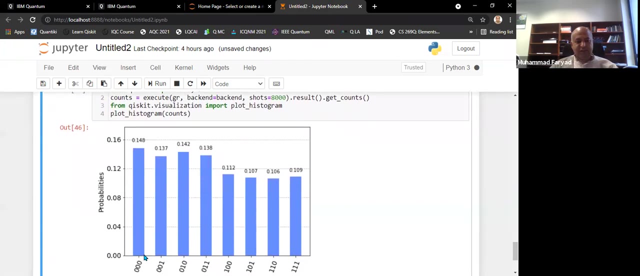 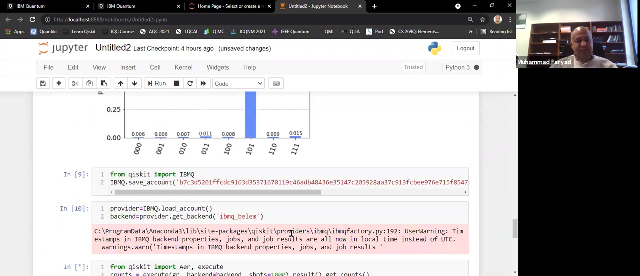 so ibmq vellum, okay, i have submitted the job and you can see my results from previous simulations on kyoto that i ran and they're almost all garbage. uh, it couldn't tell me, okay, which one is solution. space, and one reason is this: that the circuit that we have implemented right now 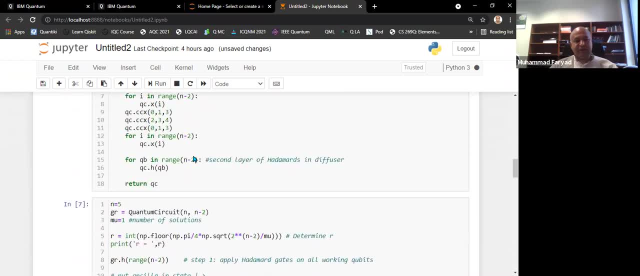 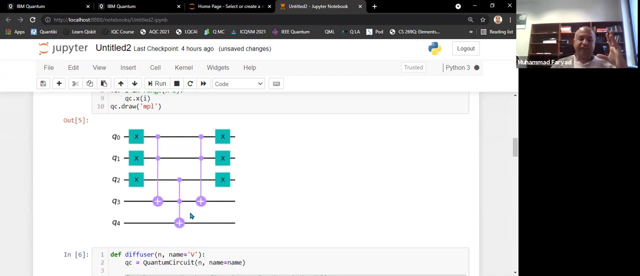 it's actually a very complicated circuit. we have implemented several toffoli gates which will ultimately have broken down to several control x gates. and control x gates are still very noisy. so, just to give you an idea, each of the toffoli gate usually uses three or four control x gates. 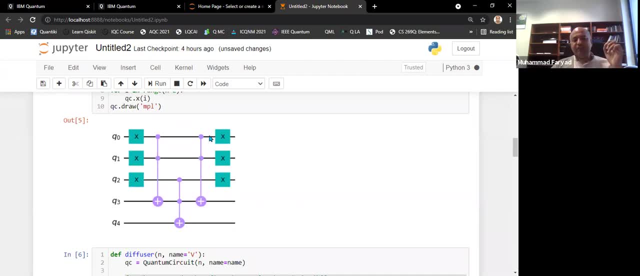 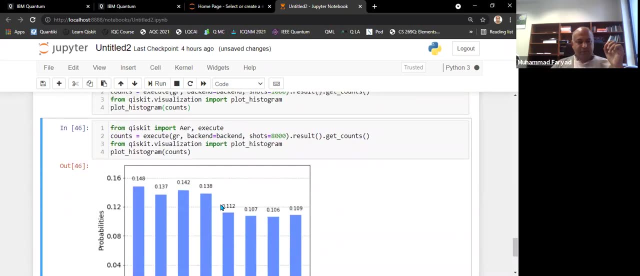 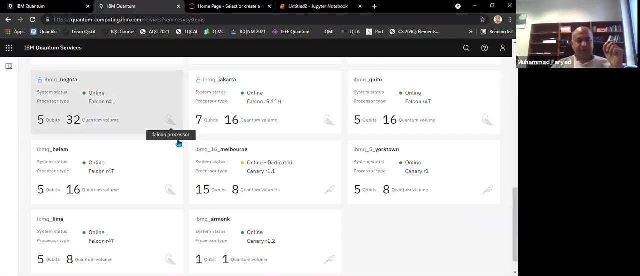 in addition to other, so this is actually a very- you know- big circuit that is just looking like a very small circuit. okay, so while we are waiting for results from uh vellum, let me go back here and just show you this interface a little bit more so. 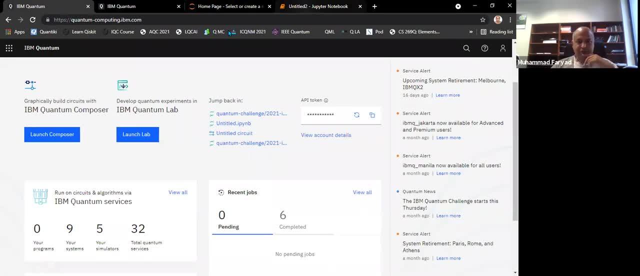 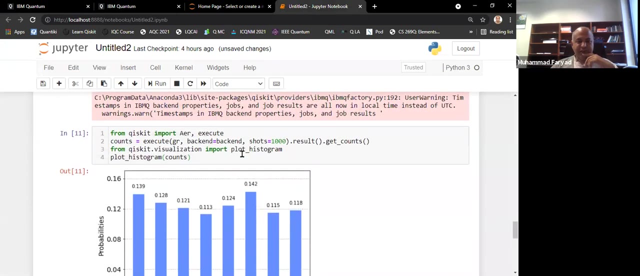 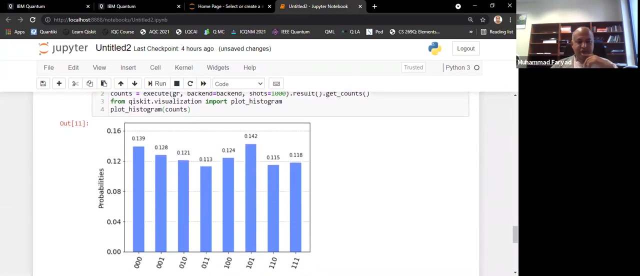 showing the result. so i still have zero pending job. is it run already? oh, yes, so we got the results back and we were supposed to have a 101 as our answer, but unfortunately 101 still has, you know, high probability than the other one, but not that high that we could unequivocally say that, okay, 101 is the solution. but anyway, this is the. 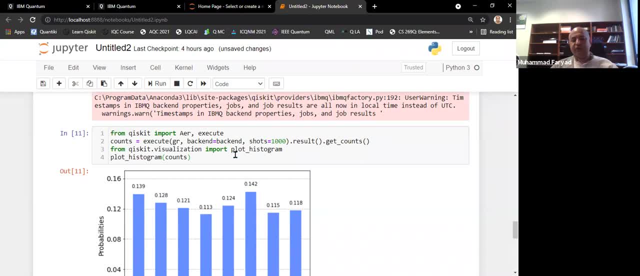 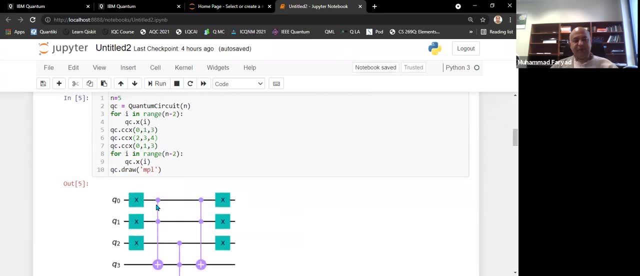 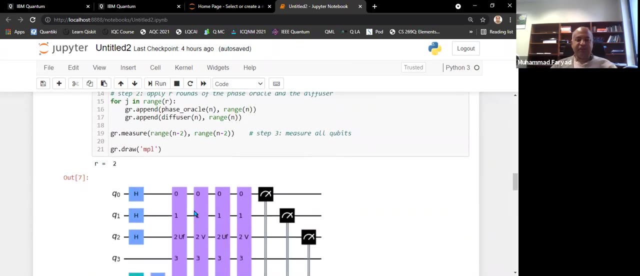 problem of running programs on quantum computer that have you know higher number of these gates, because this toffoli is implemented using a lot of control x and so on and we are using a circuit that have many of these. so if like one, two, three, four, so there are anywhere close to. 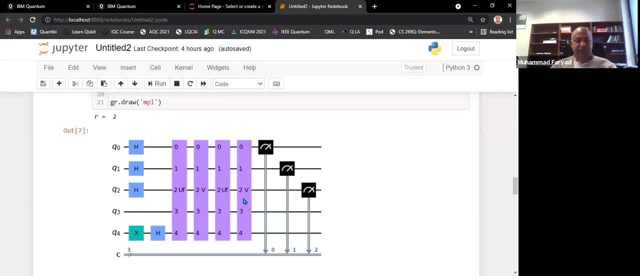 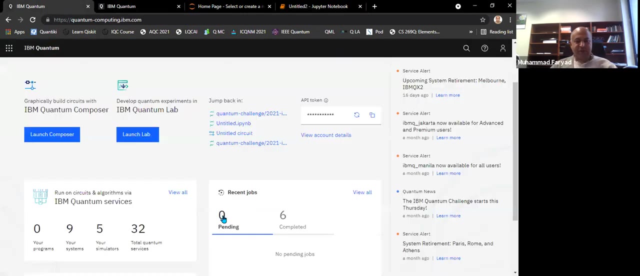 30, 12 toffolis and if you go to cx, like about close to 30 control x gates are here, which mean that this is a very big circuit which is, you know, inducing a lot of noise. we might, you know, get better result if we run it. 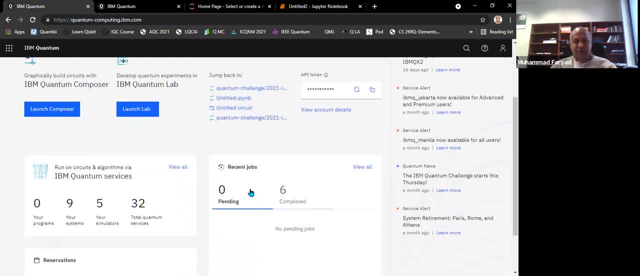 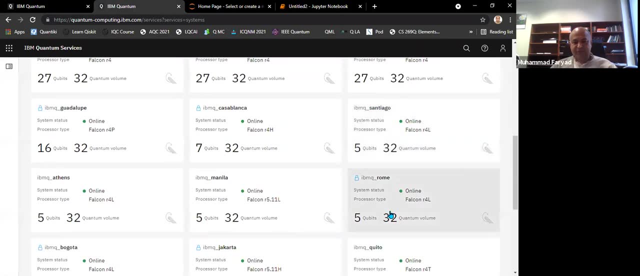 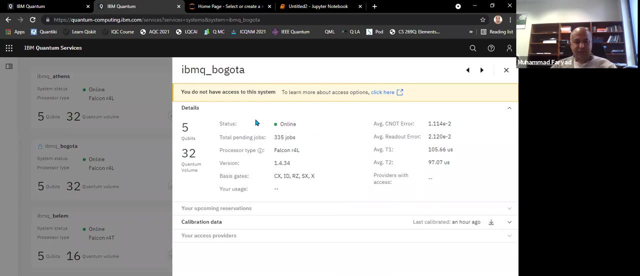 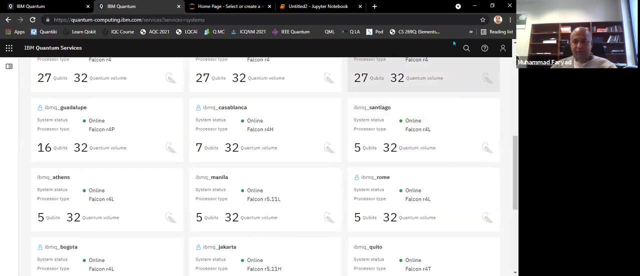 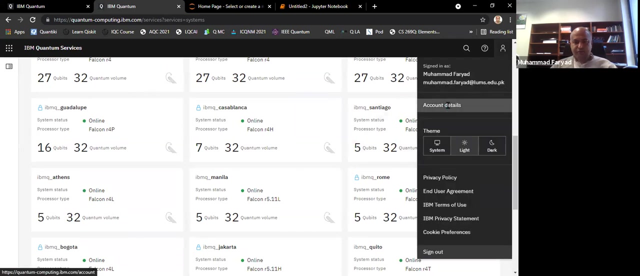 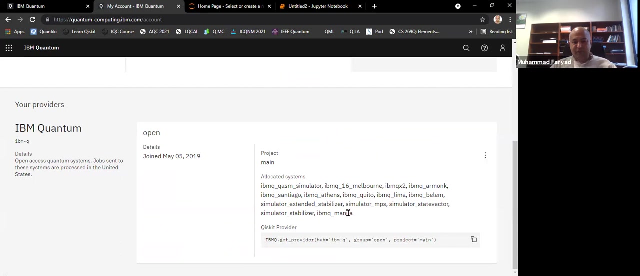 on a better quantum computer with a bit higher volume, for example this brooklyn, or. but i don't know if this brooklyn is available in free category or not, so okay, so i i, if i go to my account detail, i can see what computers are available to me. so i have manila.